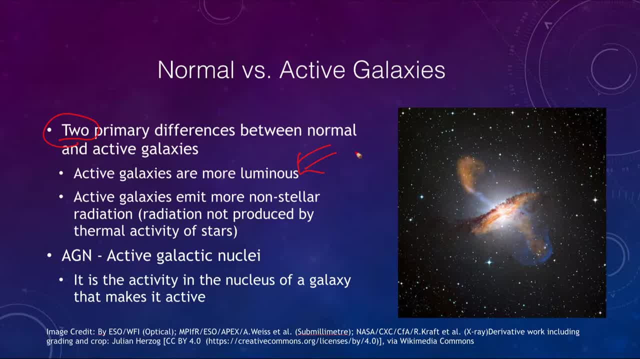 mean brighter and more luminous. Luminous does not just mean brighter and more luminous, But then also there areえ集團 of a large and waymmmelu tapa نن 911 м gas غяд нنor. 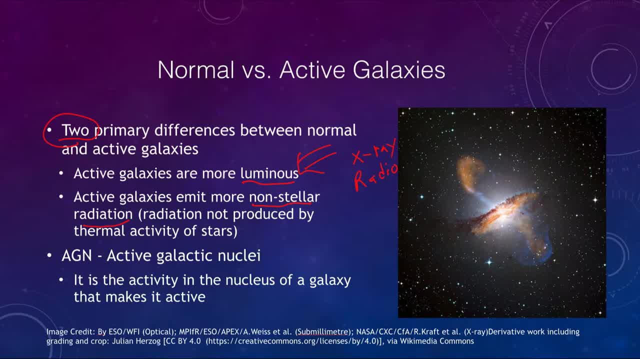 World War II크. an ordinary galaxy. its spectrum is essentially the combined spectrum of all of the stars that make it up. for active galaxies, its overall spectrum looks much different. and then we also use the term AGN, or active galactic nuclei, to talk about the activity in the nucleus of the galaxy, which, in most cases, is where 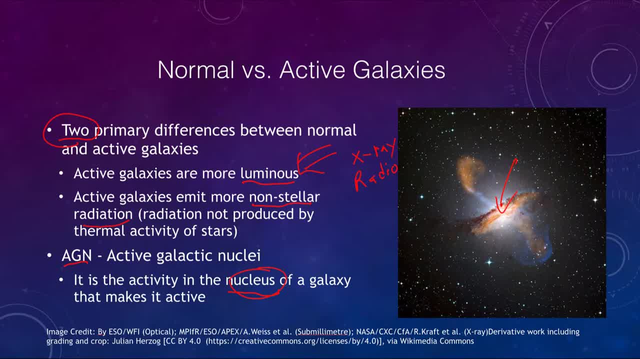 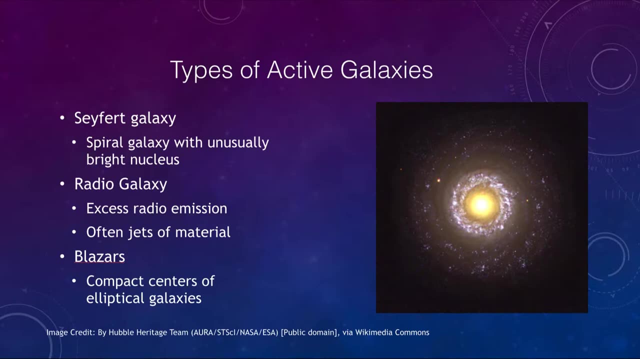 something is going on down in the nucleus of the galaxy, near the center, near that supermassive black hole. that is what is causing a galaxy to become active. so let's look at some examples of types of active galaxies. so one example of an active galaxy would be what we call a Seifert galaxy. these are: 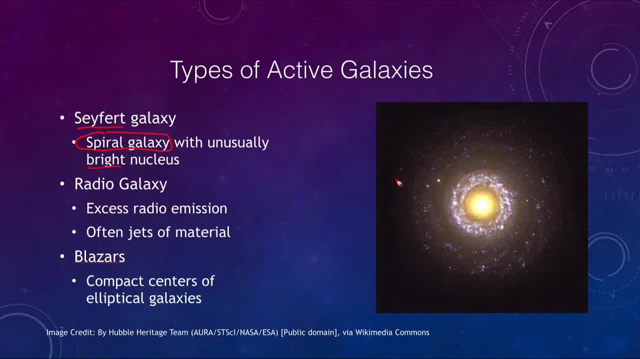 essentially spiral galaxies with an unusually bright nucleus. so what we see here for the nucleus is a lot brighter than we would normally expect for a typical spiral galaxy. that can also be called a supermassive black hole. Seiferts can often be also be associated with extensive bursts of star formation, so you can have 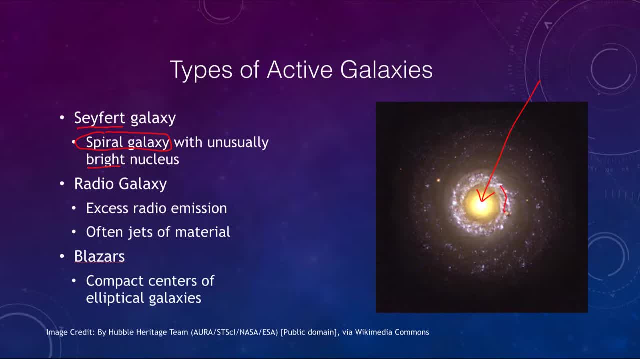 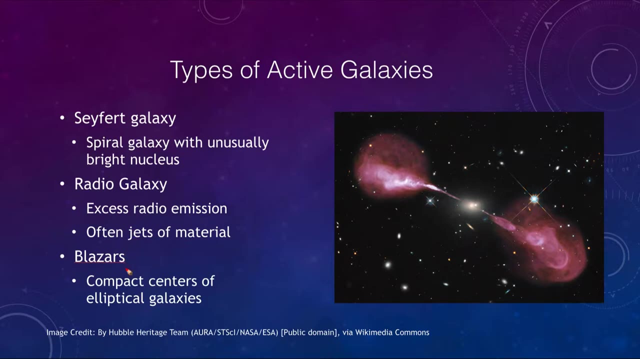 sometimes see intense regions of star formation around as well. so Seiferts are one type that are associated with a spiral galaxy. another would be what we call a radio galaxy. now, here we see the radio galaxy. they have, as you might expect, excess radio emission and often emits jets of material. so we 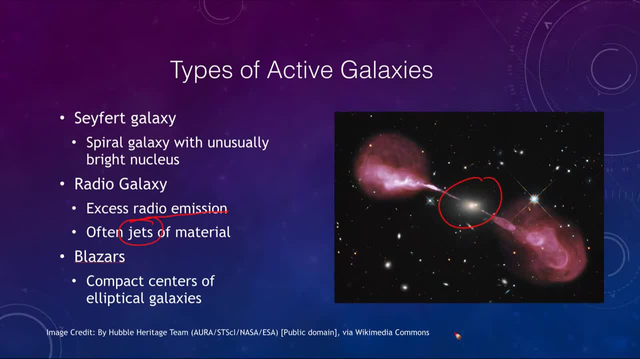 see that here the galaxy itself is down at the center. so this would be a nice- looks like a nice elliptical galaxy at the center and it is emitting a lot more radio emission than a regular elliptical galaxy and it has jets of material beaming out in each direction. you can see how highly collimated the beams are. 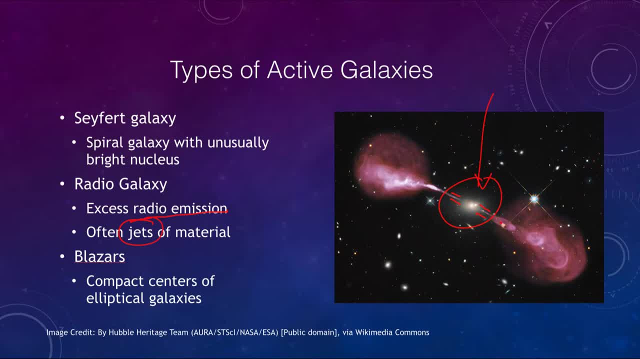 here as they leave this area and then as they reach and strike the intergalactic medium, they then spread out into these great radio lobes. So this is actually a combined image looking at a couple of things, in that you can see the optical emission but you can also see the radio emission from the 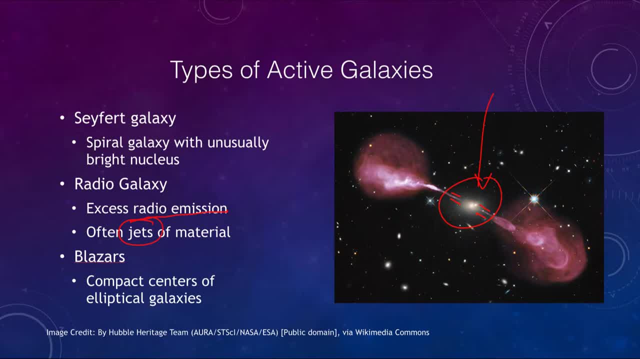 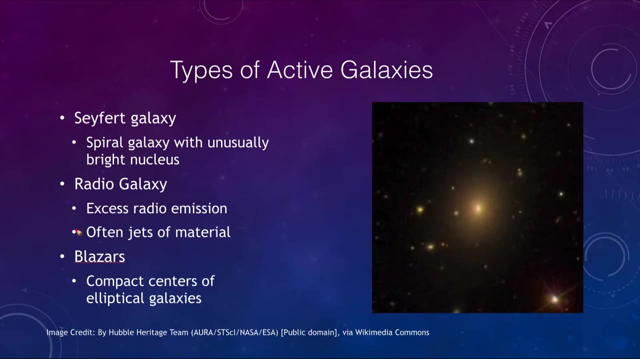 jets plowing into material in between the galaxies. and when we look at the centers of these, the other thing that we'll see is that we call what we call a blazar. Now, a blazar is actually a, the compact center of the galaxy. So when we see them, they are considered the central portion, so the very compact. 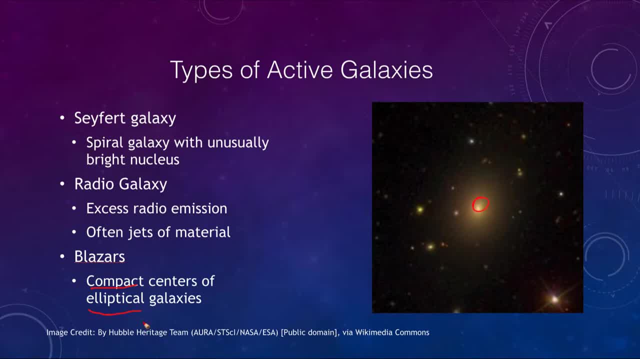 material going on at the center of, in this case, an elliptical galaxy. So what we're beginning to see is that certain types of galaxies, certain types of active galaxies, are associated with certain type of normal galaxies. Seifert galaxies are an example of a spiral galaxy, whereas the blazars are related. 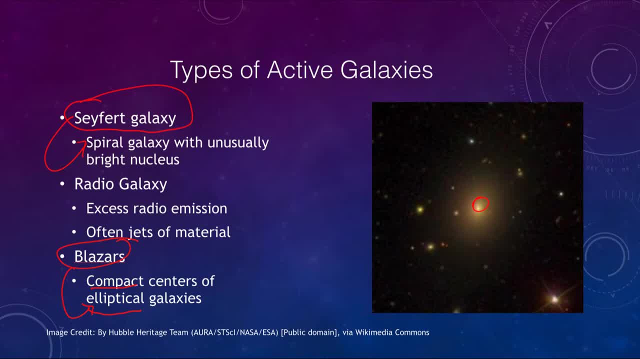 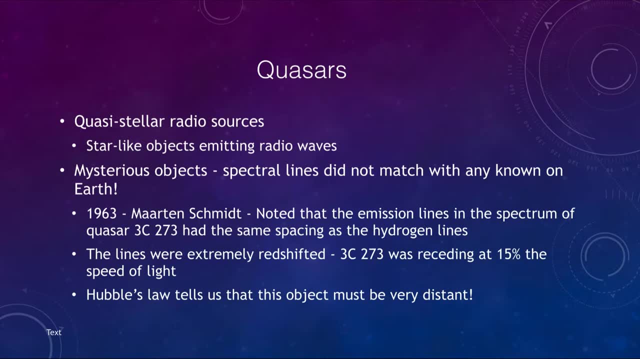 to the elliptical galaxies Now the one we really want to look at here and take some time on is the quasars. So quasars are what we call a quasi stellar radio source, and they are essentially a star like object, meaning they look like a star, they just look like a point of light, but they are. 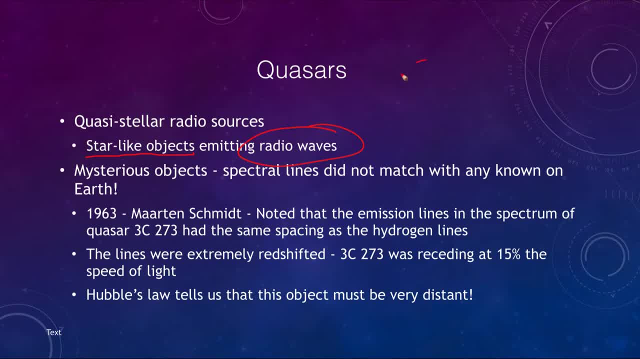 emitting radio waves. Now, that's not unusual. our Sun does emit radio waves, but we can only detect them because we are so close An ordinary star we would never be able to detect it. even within our galaxy, we would not be able to detect it emitting radio waves. So this was something very mysterious as to 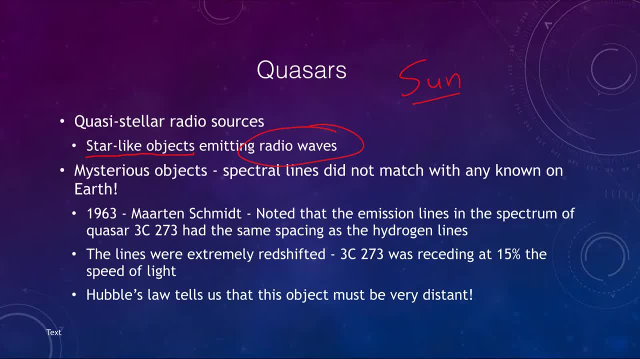 why these stars were emitting radio waves, And the other issue was that the spectral lines did not match with any that were known here on Earth. What were these things made up of? Their spectral lines did not match with what we saw here on the earth. And in 1963, Martin Schmidt 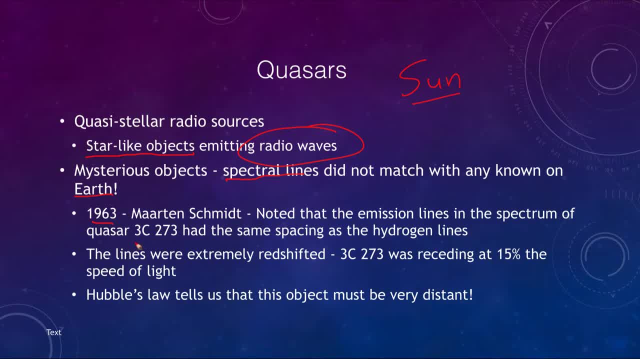 noted that the emission lines in the spectrum of a quasar known as 3c 273 had the same spacing as the hydrogen lines, but they were extremely redshifted- not just slight redshifts but an extreme redshift, and in fact enough to show that. 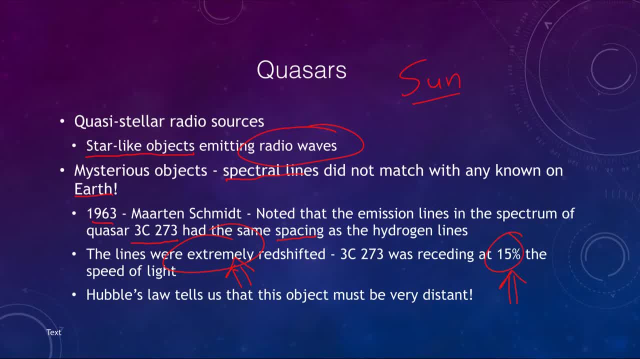 it was receding at 15% the speed of light. So that is extremely fast, much faster than any star is moving and much faster than the galaxies that had been used at the time, seen at the time, were moving. So if we use this we now have, we can use Hubble's. 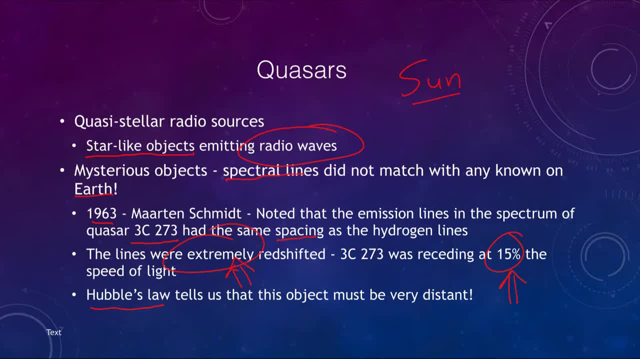 law which says that the velocity is equal is related to Hubble's constant times, the distance, and that means this object must be extremely far away to be receding at such a great speed. So what are these quasars? Well, let's take a look here, and they are star-like. 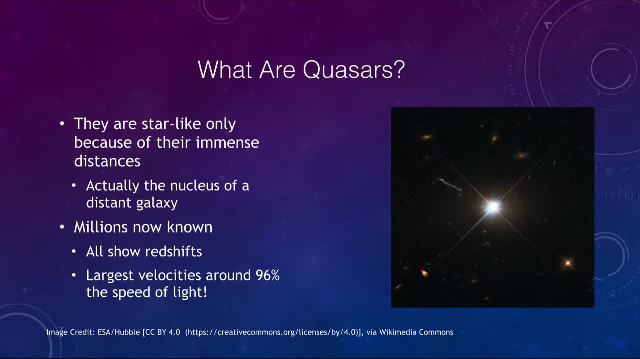 and we see here it looks much like a star. A galaxy normally has some kind of extended structure to it. We see a couple examples of galaxies here and they do not show the diffraction pattern, the cross-like pattern that we see, that goes through the center of a. 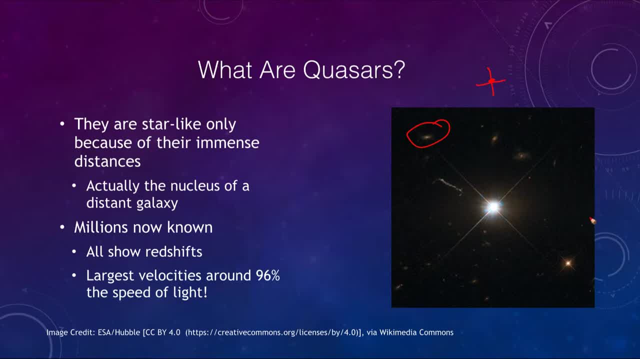 star caused by the telescope that is observing it, So that is normally associated with the star. So we'd look at this and would say, well, this is a star, it is a point source of light, but they are only star-like because they are so far away. This is actually the nucleus of a distant 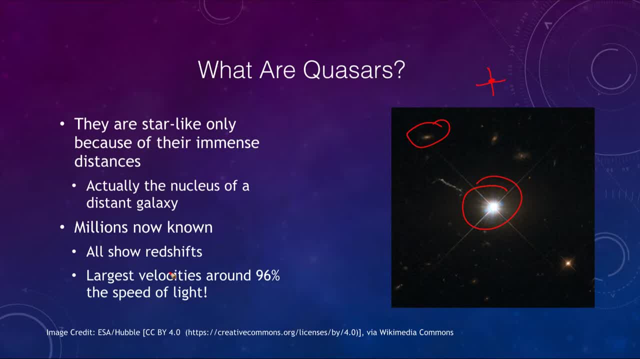 galaxy blazing incredibly bright. We now know of millions of these. Every single one of them shows a redshift, and they now have velocities going up to 96% the speed of light, Meaning that these are things that existed very early in the history of our universe. 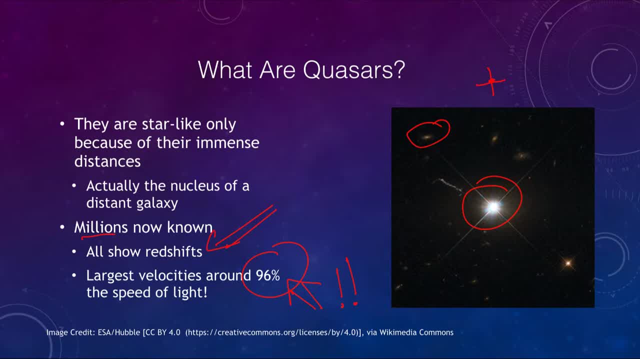 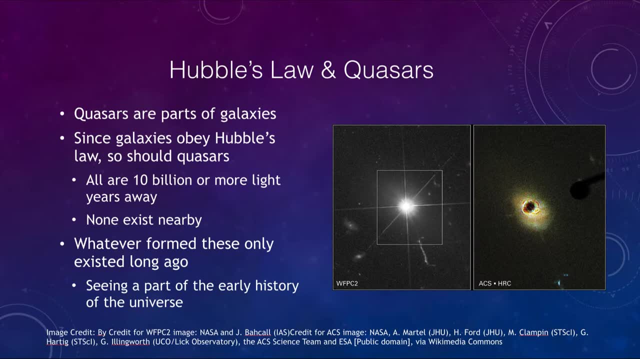 Let's take a look at some of these. Let's look at what this means from in terms of Hubble's law, and what we see is that quasars are parts of galaxies. So since galaxies obey Hubble's law, so should the quasars, And that means that, based on the measurements that we make, 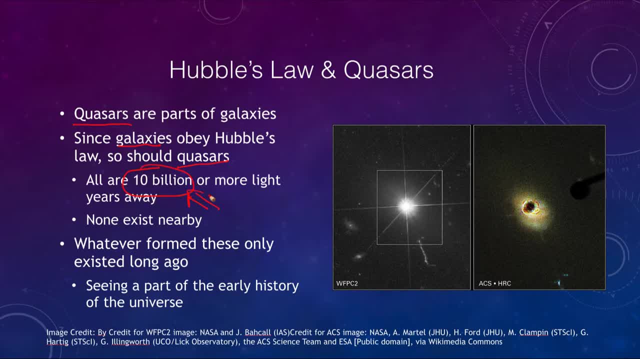 every single one of these is at least 10 billion light years away. Our universe is 14 billion light years away, 14 billion years old, So these things are really the very first couple of billion years of the universe. There are none of them nearby. There are other types of active galaxies that 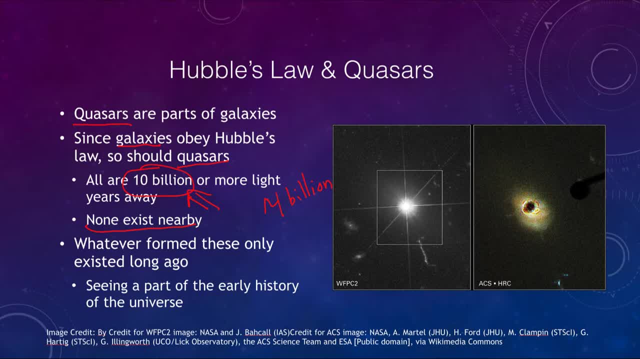 we looked at, but nothing that matches what we see for a quasar, So whatever formed, these had to have only existed long ago, and this is a way to look at the early history of our universe. We are actually seeing, then, the early history of our universe. 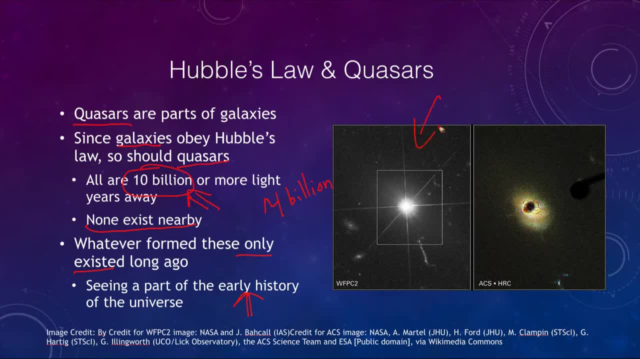 So here is an example: when we take an image of one of these quasars and look in more closely and if we blot out the quasar light, we can actually see that there is a galaxy around there as well, Just much too faint to normally be seen. So there is actually a galaxy, This. 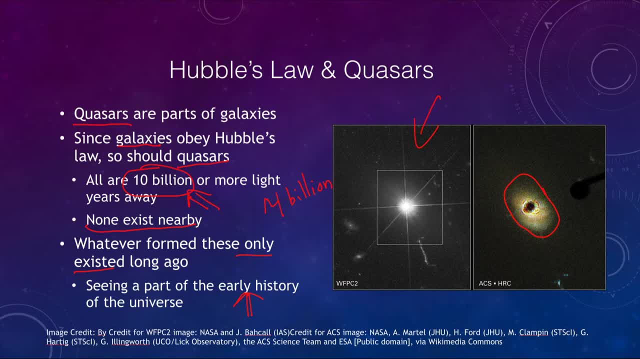 is the core of the galaxy, But if the galaxy, the core of the galaxy, is receding at such a speed, then so will the entire galaxy. Now what we have to look at is the speed of light. We have to look at the speed of light. 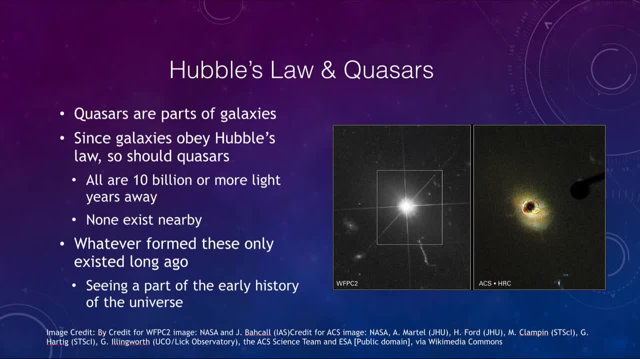 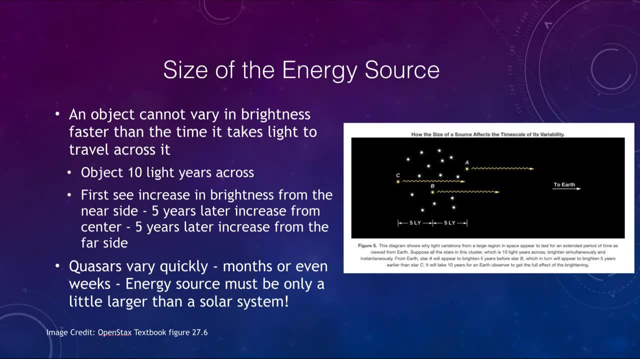 We have to look at. what is this energy source? What could be powering something to be this bright and be seen over such tremendous distances? And one thing to look at is how big this can possibly be. And what we look at is that an object cannot vary in brightness faster than 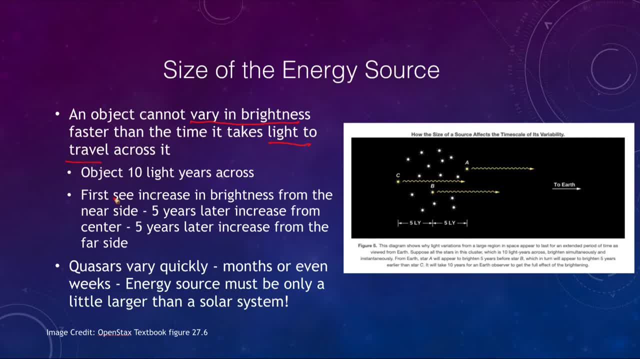 it times takes the time, the time it takes light to travel across it. If we look at an example, an object ten light years across would then? first we would see the increase in brightness from things on the near side. So if this is a cluster of stars or an object, and looking at each of these different parts of this object, 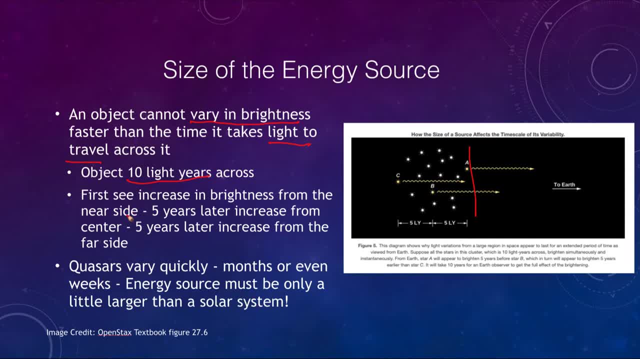 If it were this big, we would get the near side. we would get an increase in brightness. Then, five years later, we would get an increase in brightness from the middle and ten years later we would get the increase in brightness from the far side. So the increase in brightness. 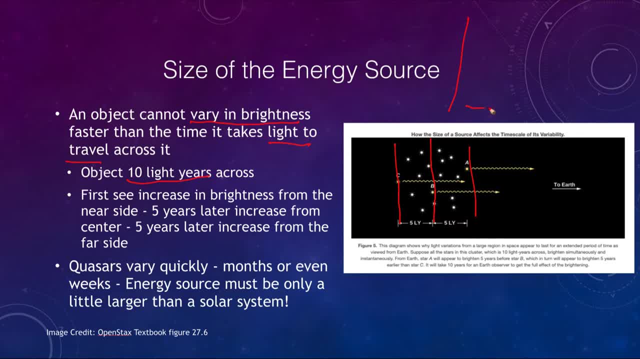 instead of just jumping up really fast. take a much longer time to increase its brightness, because it takes time. Even if the whole thing got brighter at once, we would not know about it for 10 years, Five years. we'd learn out the first side. 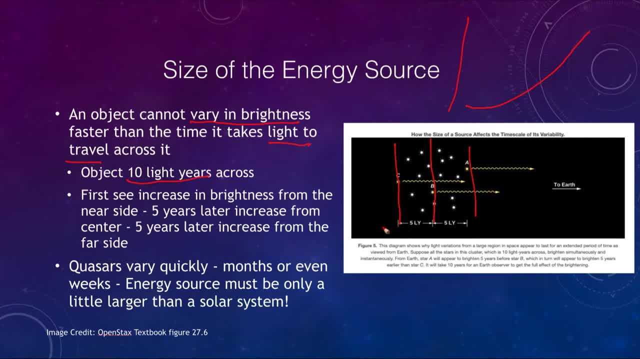 Five years later the next side, Five years later the end, And then it would continue to vary in brightness. But quasars can vary with time periods of months or weeks. That means these things cannot be light years across, They cannot be galaxy size. 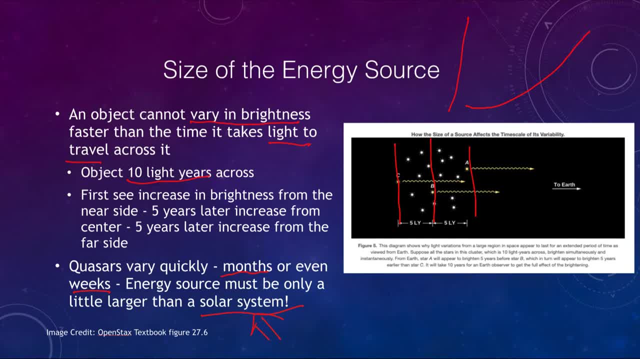 They must be closer to solar system size, And what that means is: what is the energy source of these quasars, What is the only thing that could possibly produce this much energy in such a small space? And that is where we're going to come back. 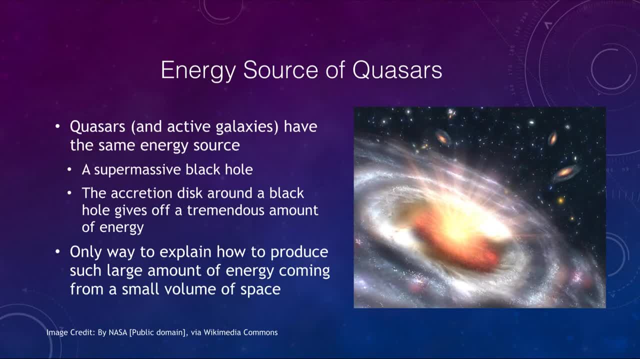 to the idea of a supermassive black hole being the energy source for a quasar, And quasars and active galaxies both have the same energy source. which is this supermassive black hole? What it is is the black hole here at the center. 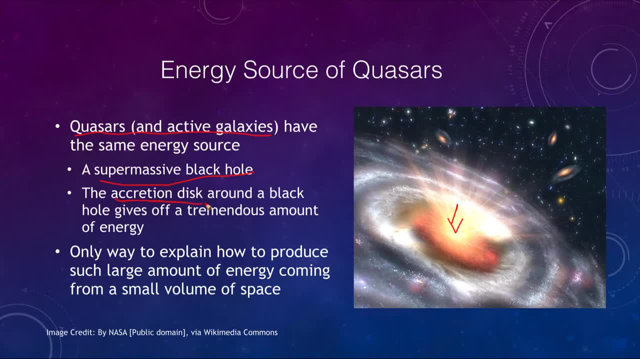 accretes material, So that accretion disk is where all the energy is coming from. So as material spirals around and into the black hole, it heats up to extremely high temperatures and gives off lots of energy. We can convert a good fraction of the mass. 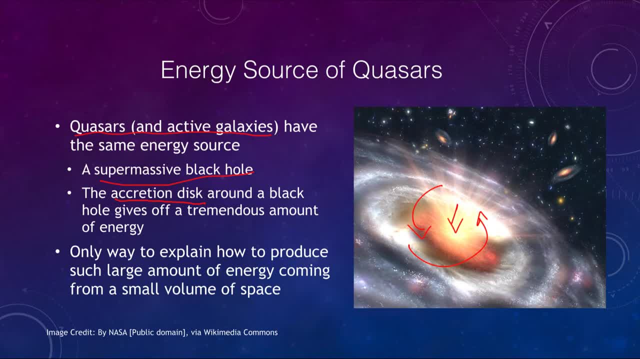 into energy in something like this, before it actually spirals into the black hole. This is the only way we have to produce such a large amount of energy: lots of energy from a small amount of space. So we have lots of energy coming from a very small space. 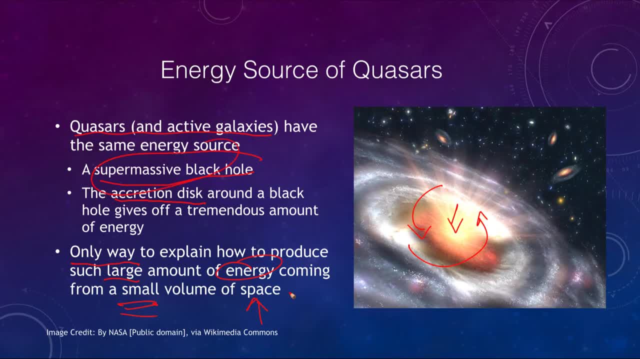 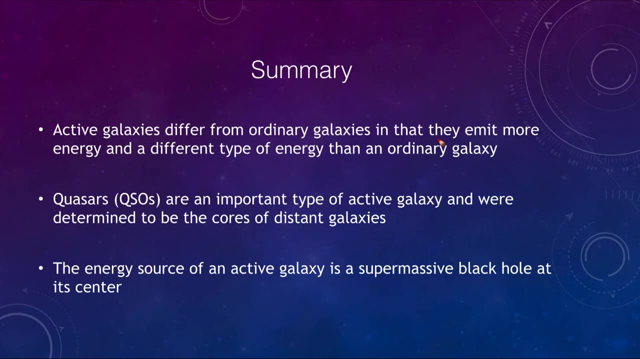 The only thing we know that will do that is this supermassive black hole. So let's finish up, as we do, with our summary and what we've looked at in this section. First of all, we saw that active galaxies differ from ordinary galaxies in two ways. 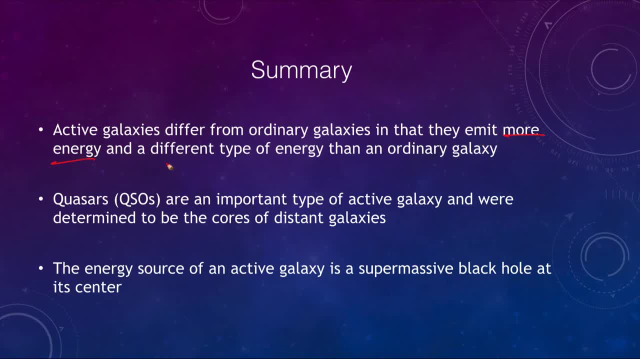 They emit more energy, So more energy coming from them, And it's a different type of energy. It is non-stellar energy. Quasars, sometimes called QSOs, are important type of active galaxies and have been determined to be the core.